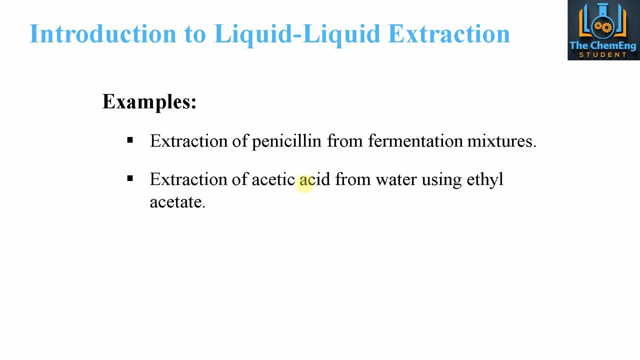 So here we can see that the acetic acid would be our solution. the water would be the solvent within this two binary mixture. We would then use Ethyl Acetate as our recovery solvent in order to dissolve the acetic acid away from the water. 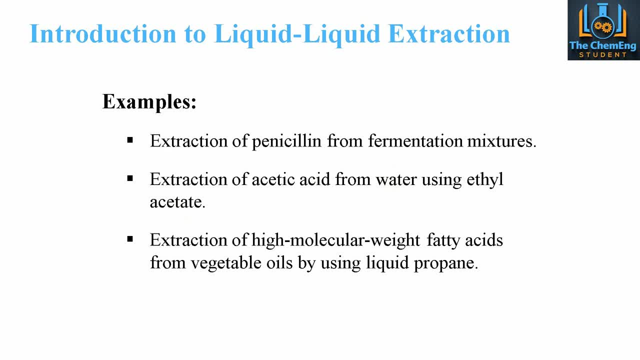 And then another example would be the extraction of high molecular weight fatty acids from from vegetable oils by using, say, liquid propane. Another example of this could be the removal of lipids from microalgae through the use of, say, hexane or other alkane or cycloalkane compounds. 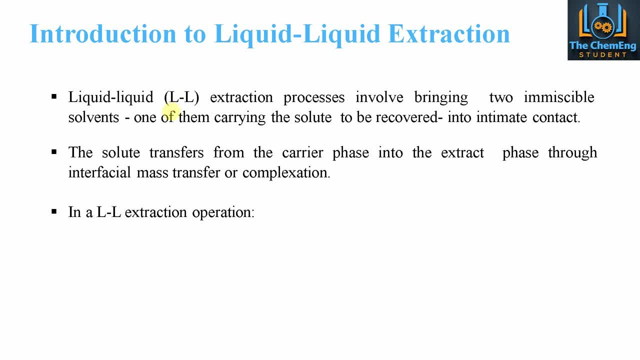 Now liquid-liquid extraction, abbreviated to LL extraction, essentially involves two immiscible solvents, one of them that carries a solute to be recovered into the intimate contact area. Now the solute transfers from the carrier phase into the extract phase through an interfacial. 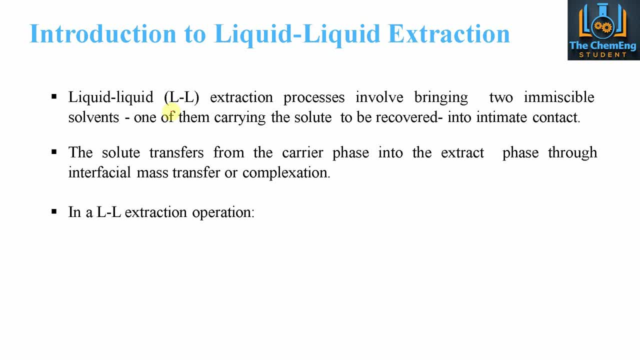 mass transfer. Now, the jargon here will look or seem fairly complex, but we will have a diagram that should help you understand how this actually works. Now, within liquid-liquid extraction operation, we have some nomenclature that we want to clear out of the way. So the solution, which is to be: 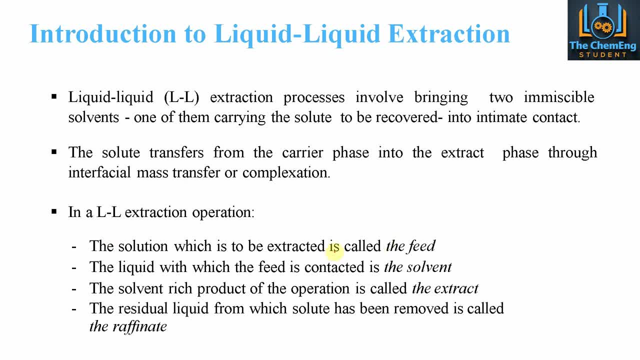 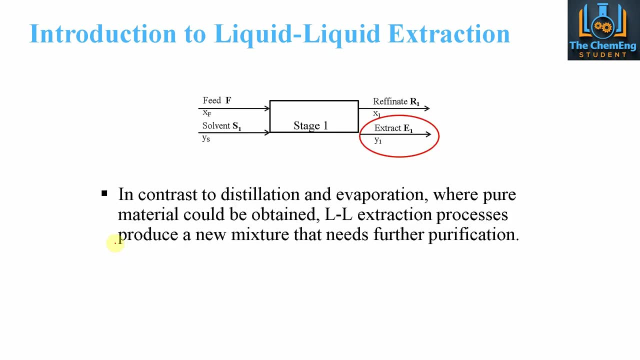 extracted is known as the feed. The liquid in which the feed is in contact is going to be your solvent. Now the solvent-rich product of the operation is called the extract, and the residual liquid from which the solute has been removed is known as the raffinate. Now a typical schematic for a single 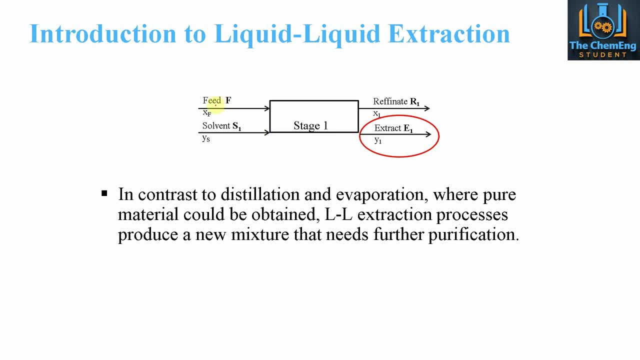 stage system would look something like this: So we have our feed and our solvent that come in contact with each other. Now, this is a co-current system because what we have is the feed and the solvent are coming in at the same point, So normally your columns would have several different stages, so we do have subsequent lessons. 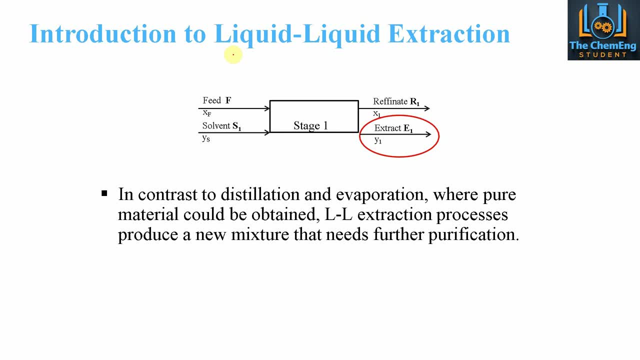 on multi-stage liquid-liquid extraction processes. So I'll put a link in our unit operations course which goes into the details of all this chemical engineering stuff. Now, in contrast to distillation and evaporation, whereby pure material can be obtained, the liquid-liquid extraction process produces a new mixture that will then need further purification. 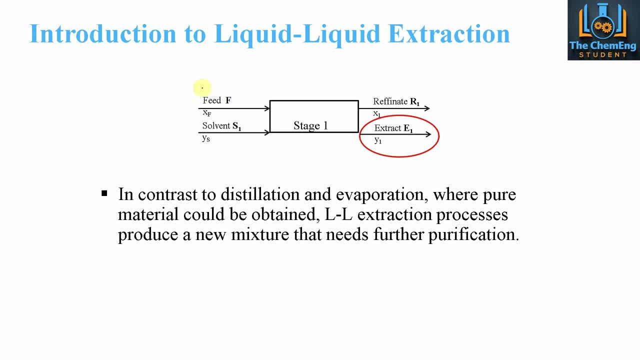 So the question would be: what is the point? because we already have a mixture that contains a solvent and a solute, Why would we dissolve another solvent to extract the solute? We're still left with our same paradox: that we have a solvent with the 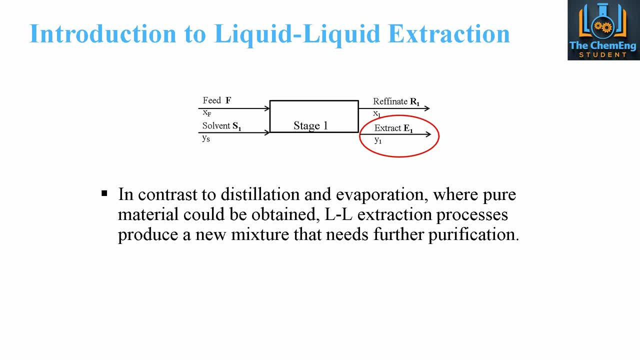 solute that we want. Well, the point here is that the solvent will be selected so that the purification process is easier to be carried out than the original feed mixture. So that is the point Now. a basic prerequisite for successful liquid-liquid extraction operation is that the 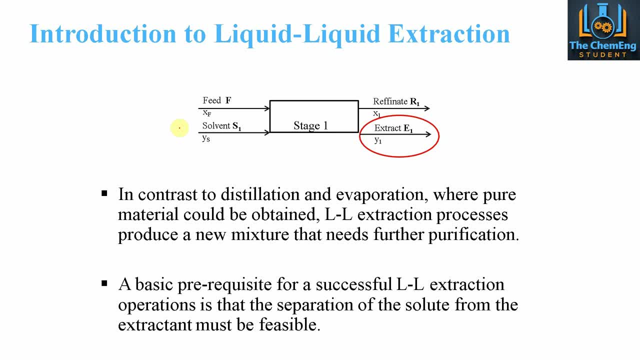 separation of the solute from the extract. it has to be feasible. So say, for example, we have an isotropic mixture here, then of course we're never going to get complete separation, Whereas if we can create a system, a new solution that can be easily extractable, then this would be. 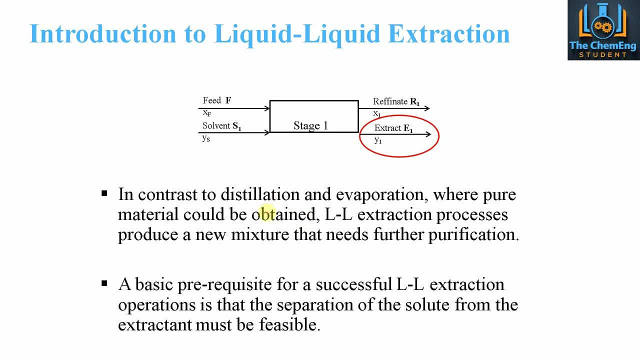 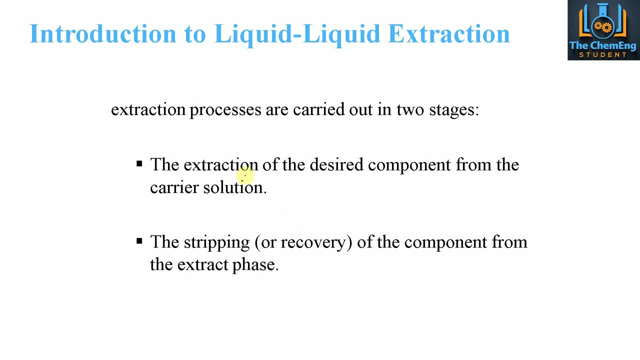 the best option. This is why we would carry out liquid-liquid extraction in the first place. Now, the extraction process can be carried out in two ways. We can have the extraction of the desired component from the carrier solution, and then we can have the stripping, or also known as the recovery, of the component from. 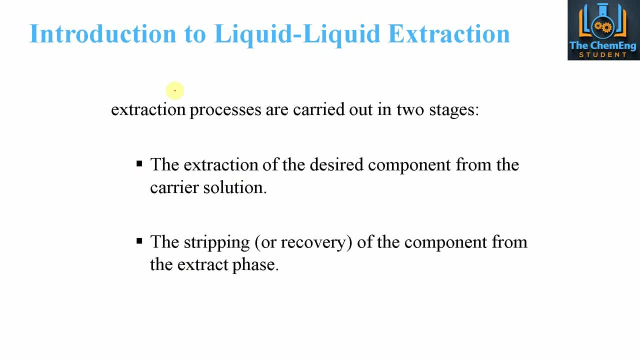 the extracted phase. So what we mean by this is your first stage here would be what we've seen in the previous slide, where we have our feed coming into the system, we have our solvent here, we will have the raffinate and we will have the extract. Now the second phase would take this: 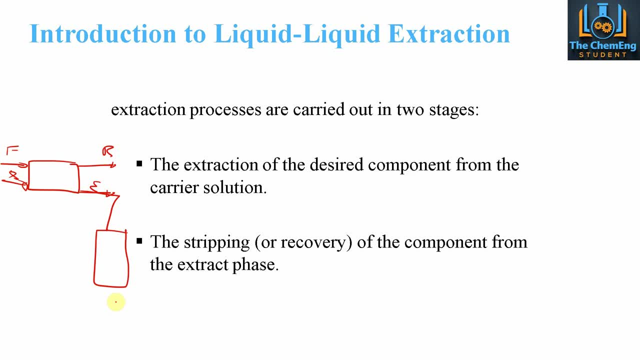 liquid-liquid extract stream, and then we would further separate it, So we could separate this through, say, a distillation column or another separation unit. So then what we would end up with is we would have our solute or our component, and then this would be the waste. 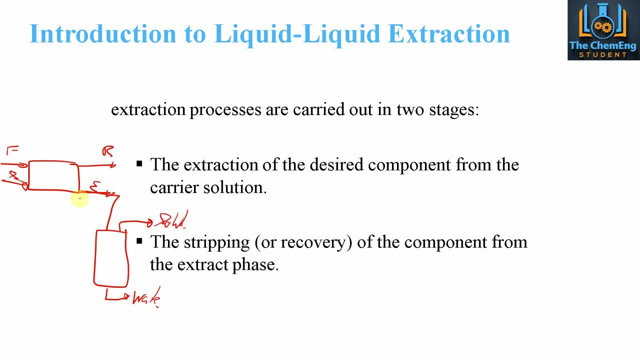 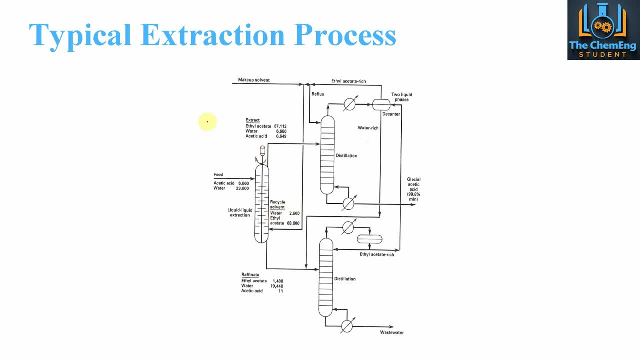 So that's a typical setup for liquid-liquid extraction. Now let's look at the flow rates. So here, what we have is we have the feed coming in, which contains acetic acid and water. Now here is our ethylene, sorry, ethyl acetate. Now these: 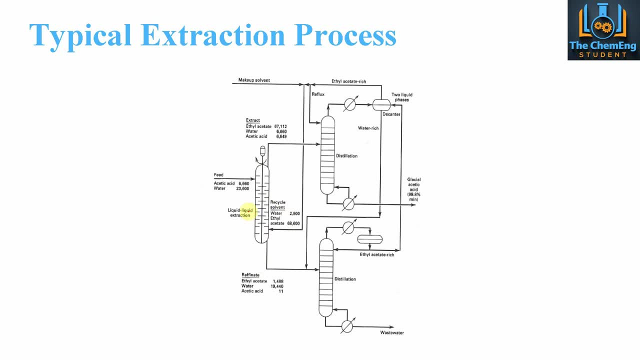 do have the flow rates. so, again, you could perform mass balances around each of these columns and check if you're getting these values. Now, if you're struggling with mass balances, we do have a full dedicated course to mass and energy balances. That's one of our more popular courses. I'll put a link in the description to that. Now, if you're struggling with mass balances, we do have a full dedicated course to mass and energy balances. That's one of our more popular courses. I'll put a link in the description to that. 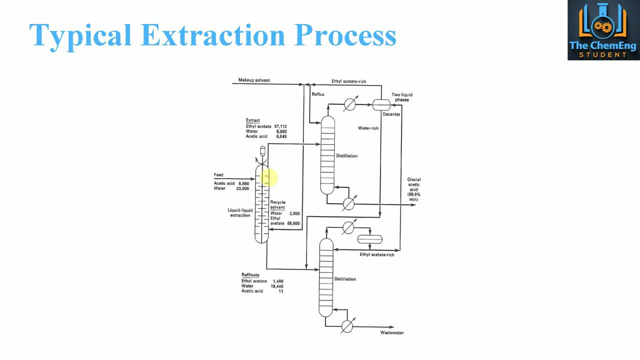 Now, if you're struggling with mass balances, we do have a full dedicated course to mass and energy balances. That's one of our more popular courses. I'll put a link in the description to that And you can check that out when you can. Now here. this is our liquid-liquid extraction column. 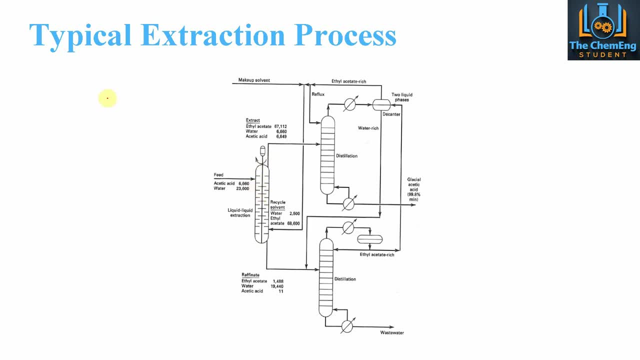 So we can see that it contains these trays, because essentially what we want is one of the liquids will fall, So we'll have this region, So this will fall. say this is the feed, And then what we would like to happen is we would have the counter current system whereby, say, this is the ethylene acid. 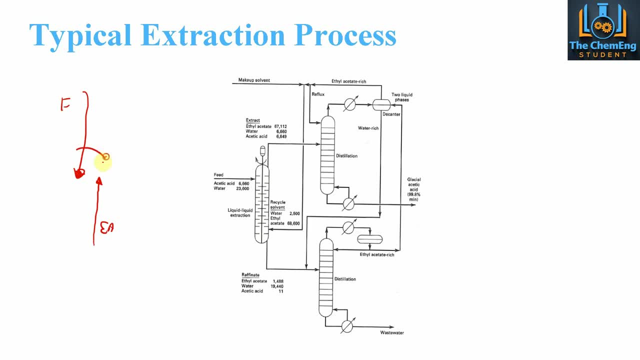 state will go in the opposite direction and the transfer of the solute will take place as they pass each other, And this here just makes the process that much more efficient in the contact area. So we're getting a better contact between our solvents and our solute. So therefore we get 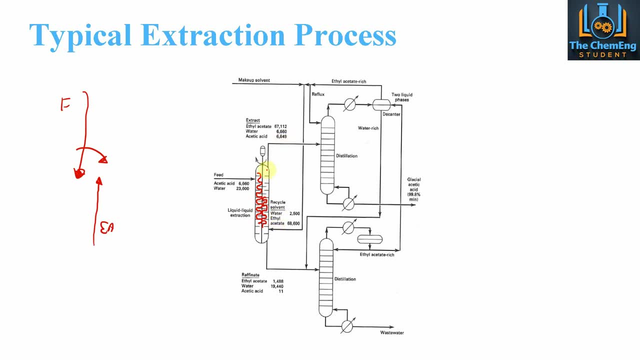 improved mass transfer. So here what we can see is that in the extract we have ethylene acetate, water and acetic acid, So we have a three component mixture. So in order now to extract this further, then what we would want to do is then place it into a distillation column. 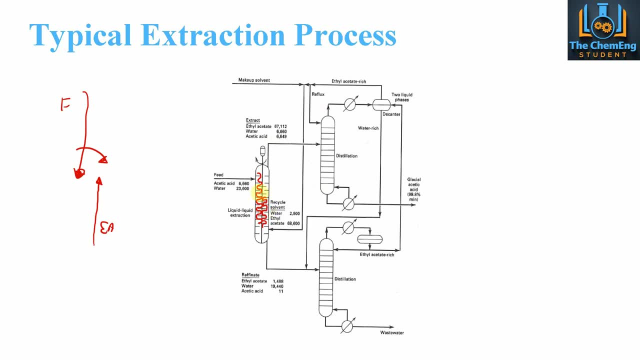 because we now know that the extraction between the acetic acid and the ethylene acetate is much easier to do. So then that's where we put it into this distillation column. We get our top product, which will essentially contain two liquid phases, and then what we can do is put this into a second. 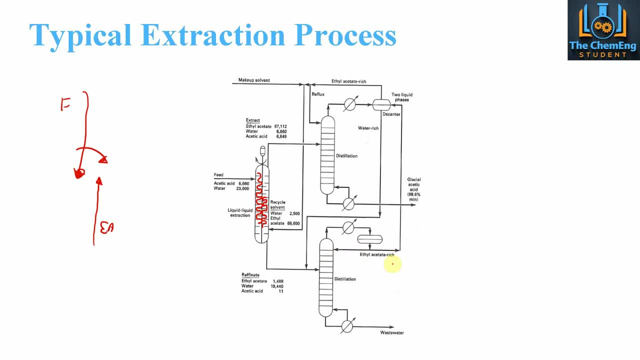 distillation column whereby we can get our ethylene acetate rich feed and we can get our waste water at the bottom of this column. Now again we can have make up solvent because we can adjust this by the reflux ratio whereby we have the recycled ethylene acetate rich. 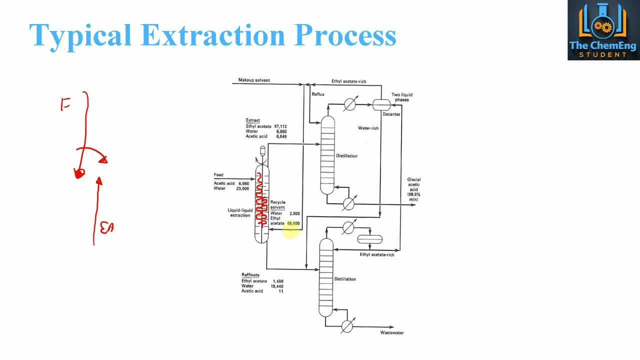 stream that we can then bring this back and then we can recycle that into the liquid-liquid extraction and the process becomes more efficient in that we are recycling our used solvent much better. So that's a typical schematic for the liquid-liquid extraction process. 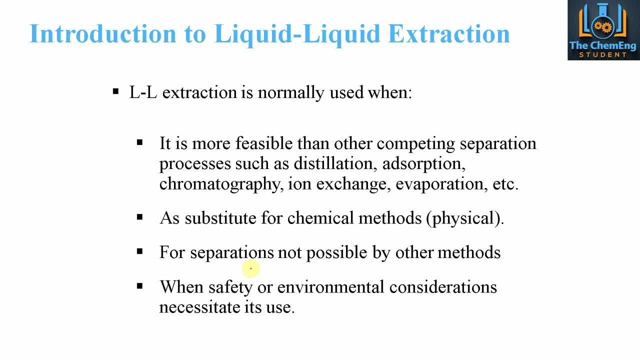 Now, allylol extraction is normally used when it's more feasible than other competing separation processes- ie distillation, absorption, chromatography- than to use these systems, because one of the key points that we made earlier was if we have, say, an isotropic mixture. 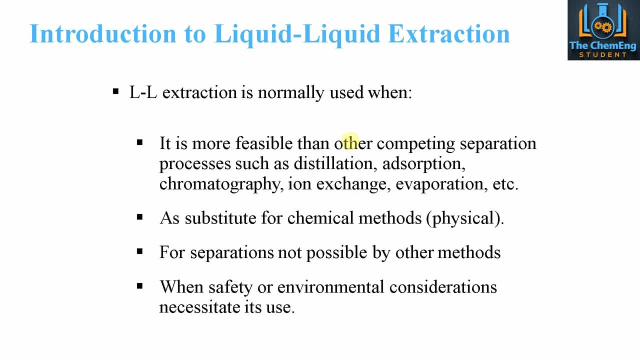 that we can't get 100% separation within a distillation column, then what we can do is try and use and manipulate mass transfer between the solute and the new solvent and then be able to separate them almost 100%. Now it's also used as a substitute for chemical methods. 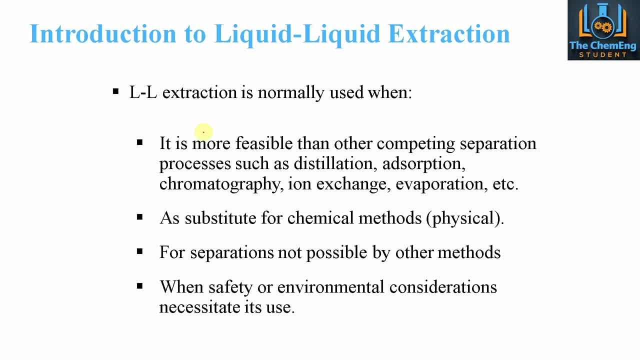 ie we can use physical methods as well, Because this is a physical process. It can also be used for the separation. if other methods are simply not going to be possible- say operating conditions, the type of component that we have- then this might be the best option. 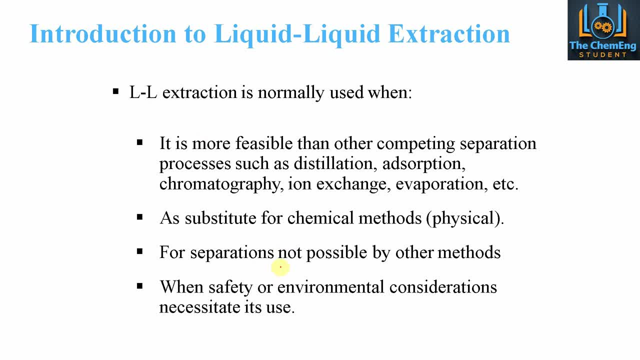 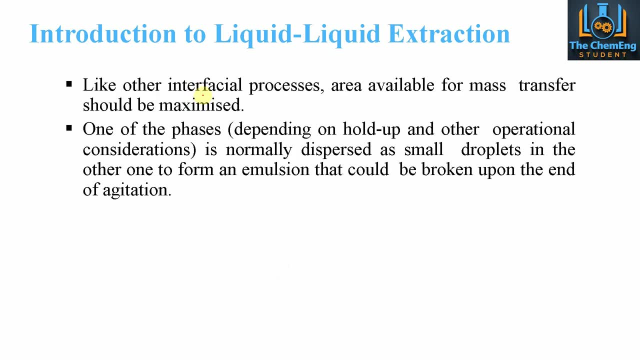 And again when safety and environmental considerations force us to have to use liquid-liquid extraction. Now, like other interfacial processes, the surface area, or contact area, must be separated. It must be maximised in order to increase and optimise the mass transfer rate. 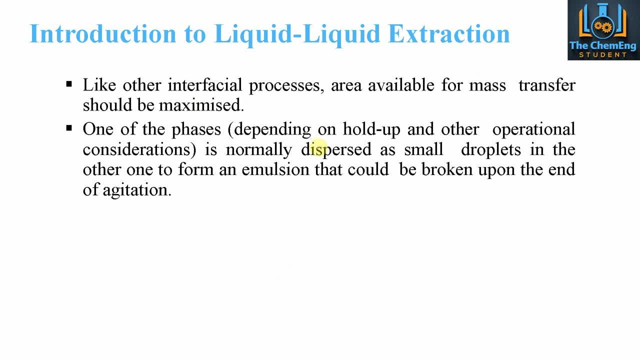 So that's why we've seen we had the different trays and the baffles in that we can separate or stretch out the mixture so that we're getting a higher contact surface area between the two solutions. Now one phase depends on the hold-up of the operation. 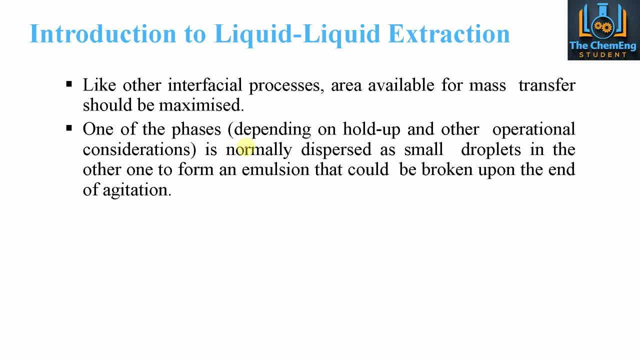 is normally dispersed as small droplets. Now, normally what you'll find is that we can. usually what you'll have is you'll have your column and say: the feed that comes in at the top, we can try and disperse that as small droplets. 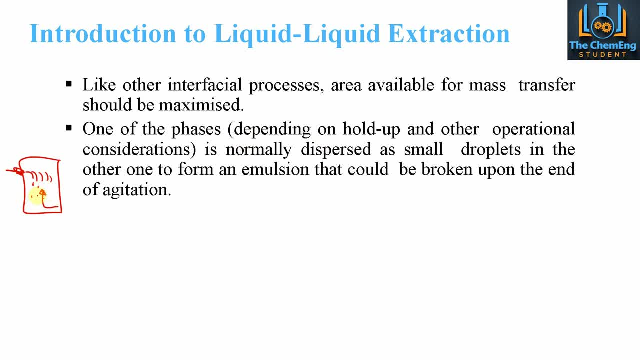 And then we can pump our other solution, so as that we're getting increased contact time And that's using spray systems. We also seen we could have the tray system as well. Now, a high surface area to volume ratio will provide the area of the solution that we want to use. 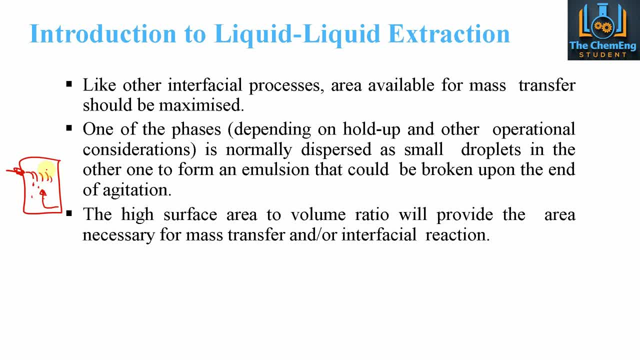 Now. a high surface area to volume ratio will provide the area of the solution that we want to use Now. a high surface area to volume ratio will provide the area of the solution that we want to use. We'll use the area necessary in order to maximize. 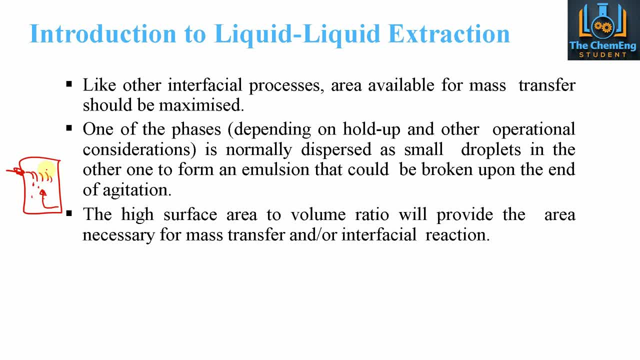 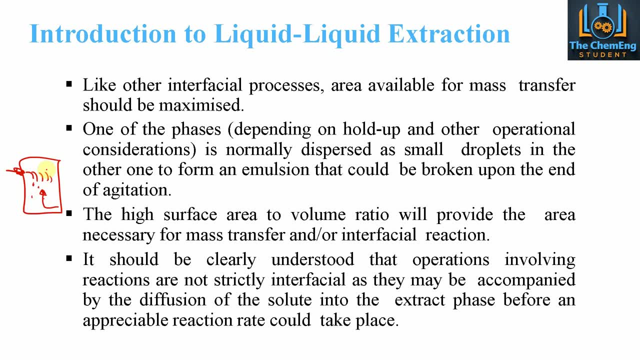 and increase the mass transfer rate and the interfacial reactions and increase the mass transfer rate and the interfacial reactions. Now it should be clearly understood that the operations involving these reactions are not a hundred percent strictly interfacial, because they can be accompanied by diffusion reactions. 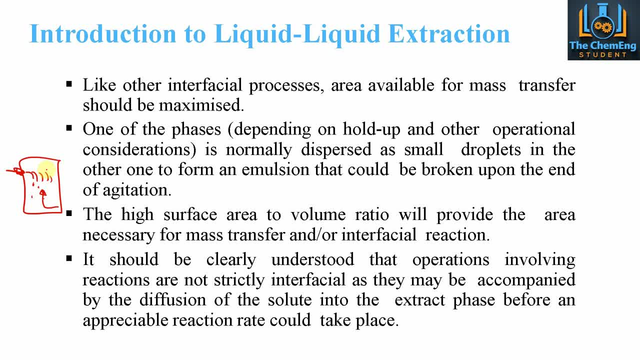 between the solute in the extracted phase before the appreciable reaction rate could take place, before the appreciable reaction rate could take place. So it's not a hundred percent interfacial. So it's not a hundred percent interfacial. interfacial we can be accompanied by some diffusion taking place, but that again we do. 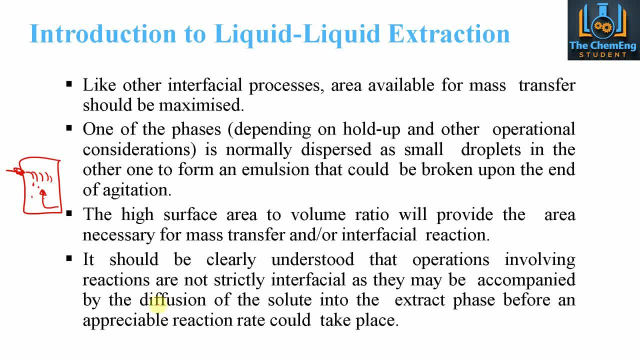 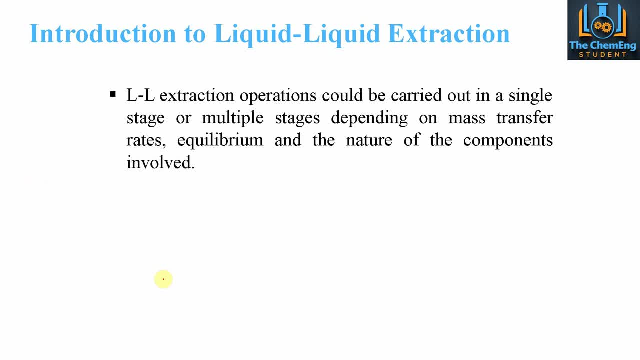 discuss that at length in our unit operations course, so if you want to know more about that again, that would be worth checking out Now. liquid-liquid extraction operation could be carried out in single or multi-stage systems. it just depends on the rate of mass transfer. the equilibrium of 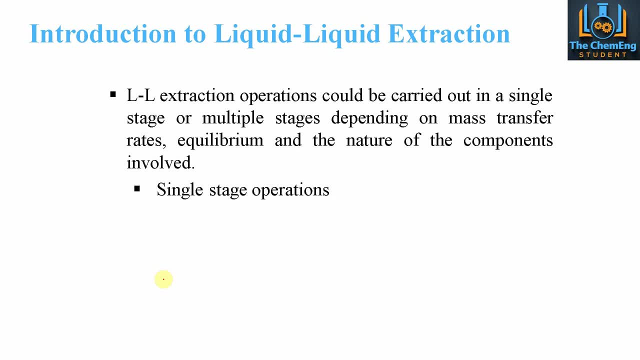 the process and the nature of the components involved. So that's where a preliminary design stage would allow us to determine if single stage operation is going to work or whether or not we need to use multi-stage operations. Granted, multi-stage operations is more intense in terms. 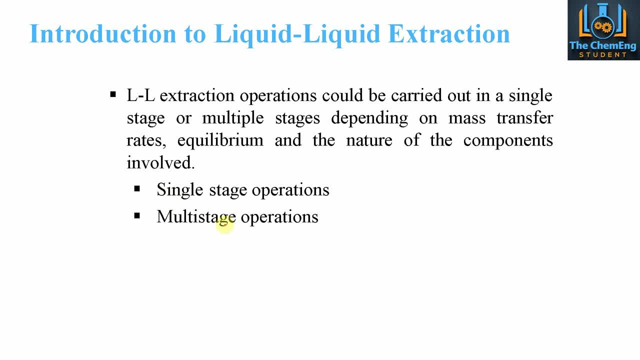 of the design, but this one can be more efficient in terms of recovery. But within each of these operations, we can have countercurrent, we can have cold current and we can also have crosscurrent contact. Now, from your background, knowledge in chemical engineering we should be familiar with. 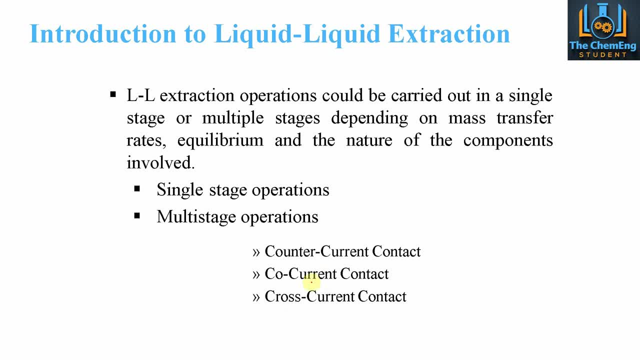 these three types of contact. you normally see these mentioned a lot in heat transfer. Now, from the knowledge based on heat transfer, we would know that the best system to use would probably be the countercurrent contact, followed by crosscurrent And then, lastly, by co-current. 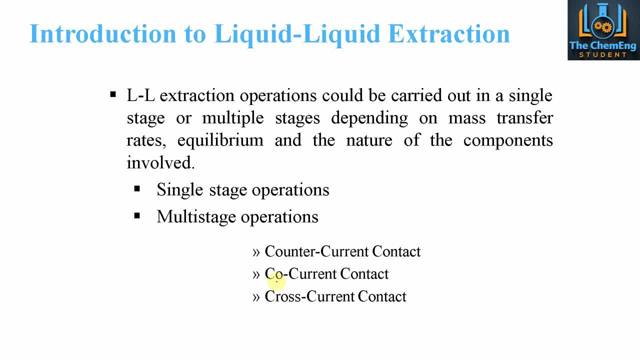 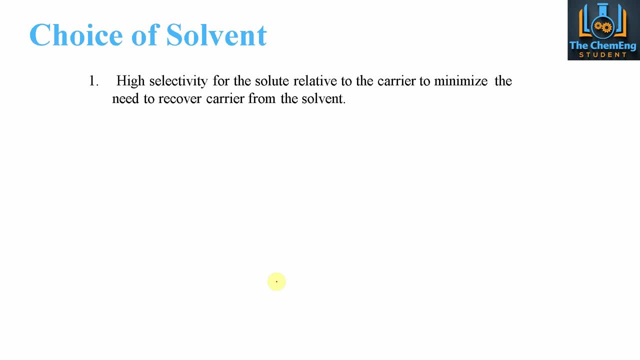 But again, this just comes down to your design. Now, as I said, the choice of the solvent is really, really important. So here are the steps that I would recommend you take in order to select your appropriate solvent. So number one is that we have a high selectivity for the solute relative to the carrier, in order to minimize the need to recover the carrier from the solvent later on in stage two. 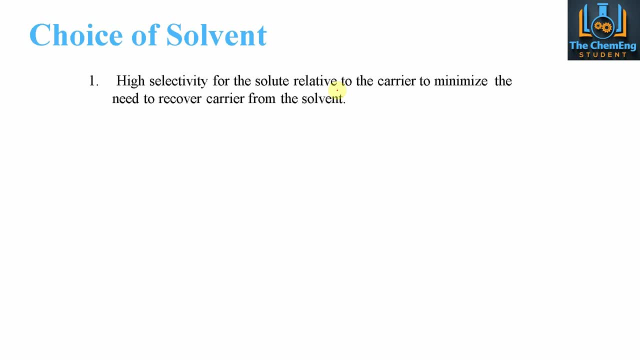 So that's key, that we want to ensure that the solvent that we pick will give easy separation during the next stage of the process. Number two would be that it has a high capacity for dissolving the solute, in order to minimize the solvent to feed ratio. 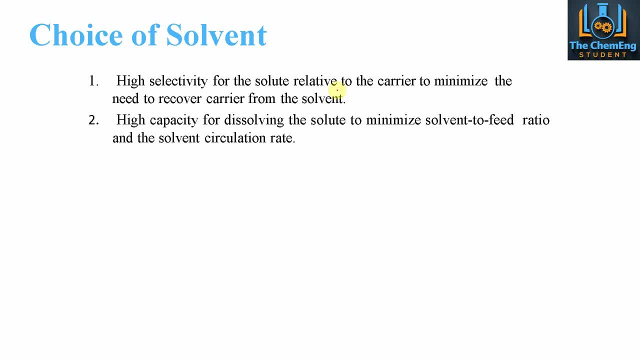 Ie if we can use a lesser volume of solvent to recover the maximum amount of solute from our feed system, then that would reduce the cost. So number three is that we have a minimal solubility within the carrier, So we need to ensure that we don't start to dissolve the solvent in our feed with our carrier solvent. 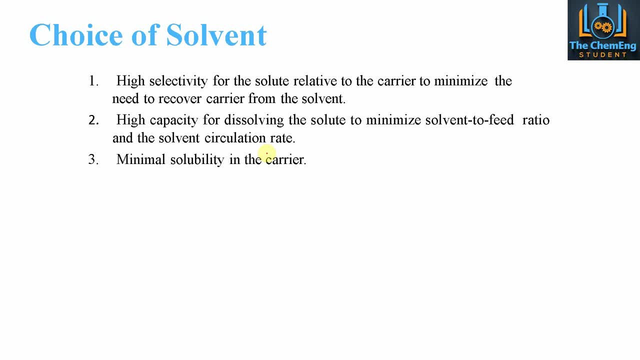 So we want to ensure that only the solute will transfer from one solvent to the other. Now we also need to account for the volatility of these components, Because the recovery of the solvent can be a significant factor. So we need to ensure that we don't start to dissolve the solvent in our feed with our carrier solvent. 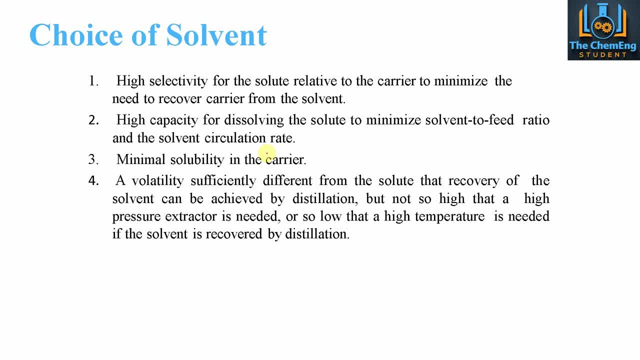 This is achieved by distillation, But it wouldn't be so high that a high pressure extractor would be needed. So therefore, low at high temperature is needed if the solvent is recovered by distillation. So what we mean by this is that if we have a high volatility, then what we could do then is we would need to use a distillation column. 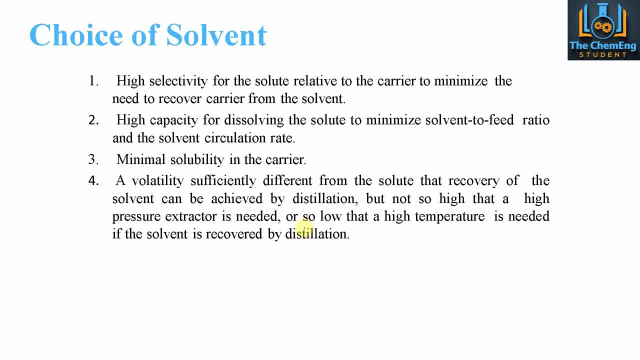 But we could use it at reduced operating conditions because we have a high volatility. Therefore, the same Separation process will be a lot easier and we wouldn't need such extreme operating conditions. Number five would be that it is chemically stable, So it shouldn't have to go an irreversible reaction within the when we receive the solute. 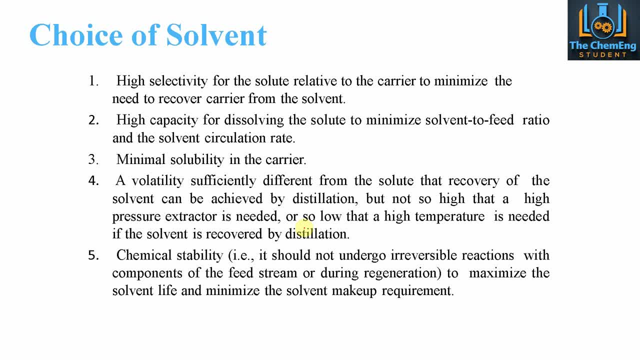 Then that would make the regeneration and the extraction even harder in the second phase. Now, this would also allow us to maximize the solvent life. And to maximize the solvent life And to minimize the solvent makeup requirements, because ultimately you want to try and reuse the solvent as much as possible. 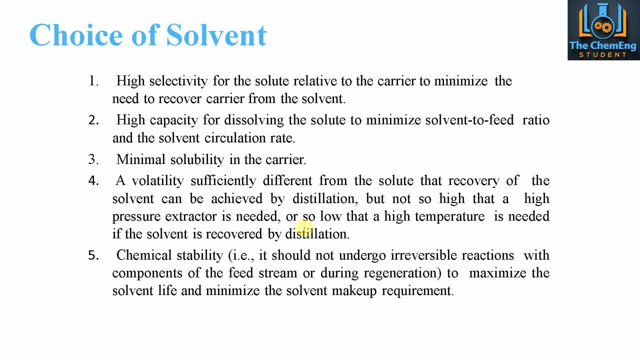 So if it continuously undergoes reactions whereby it's not as efficient as it was at the start, then we're going to have to use more of our fresh solvent, which is what we try to minimize. And then, lastly, we need to ensure that is in there in order to permit the use of common materials for construction. 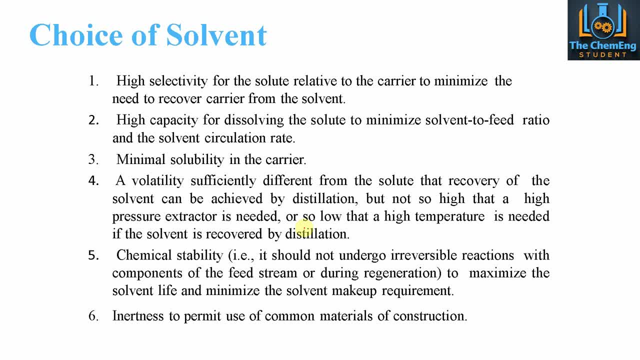 Because we don't want to use it, Because we don't want to use it, Because we don't want to use it. We don't want to create this very elaborate system whereby we have a very sophisticated carrier solvent but it is very, very toxic to our standard construction material, ie if we use stainless steel or even high carbon steel. 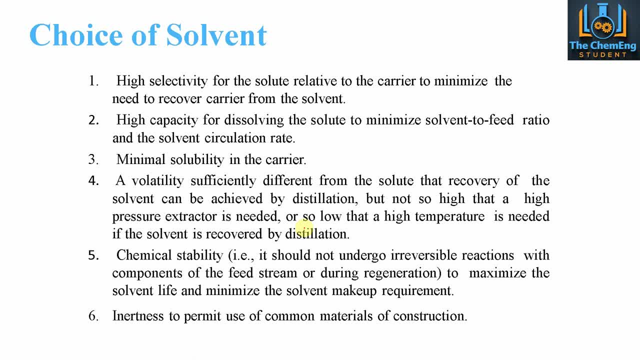